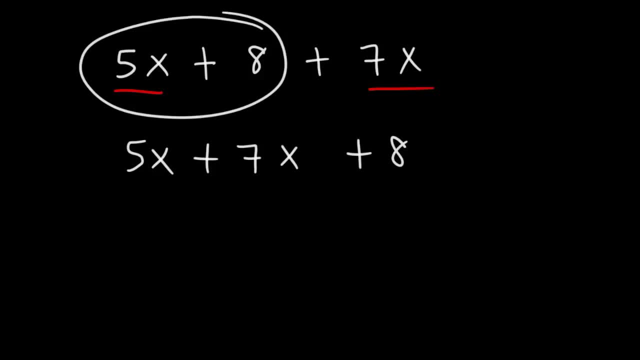 other. By the way, you can't add 5x with 8, because they're not like terms. The 8 doesn't have the same variable as the 5, so you shouldn't add them. You can't say it's 13 or 13x. That's not. going to work. Now, these are the terms that we're going to use. We're going to use the terms that we're going to use. We're going to use the terms that we're going to use. We're going to use the. 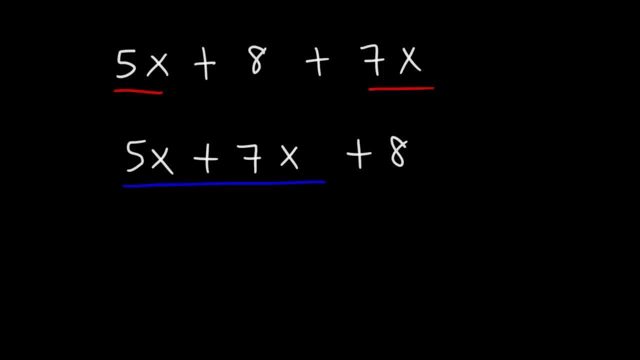 these two terms are like terms because they have the same variable x. So what we can do is we can add their coefficients to get the right answer. 5x plus 7x is 12x, So the final answer is 12x plus. 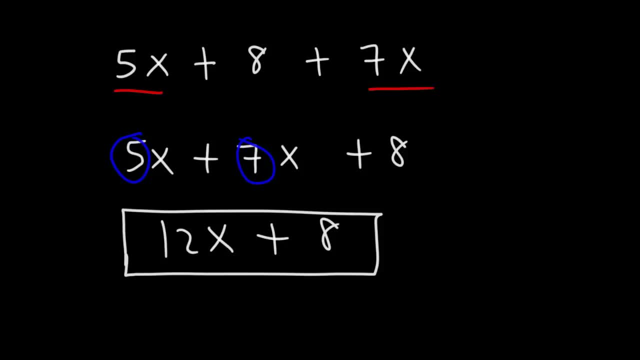 8, and we can't combine 12x plus 8 because they're not like terms. Now, for the sake of practice, let's work on some other examples. Let's try this one: 9x plus 7 minus 5x plus 4.. 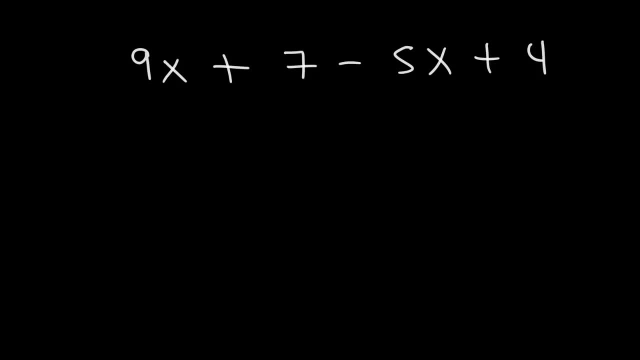 So which terms are like terms? 9x and 5x are like terms, So let's rewrite this expression: 9x minus 5x, 7 and 4 are like terms. They're both constant terms, so we can add them, So let's focus on this. 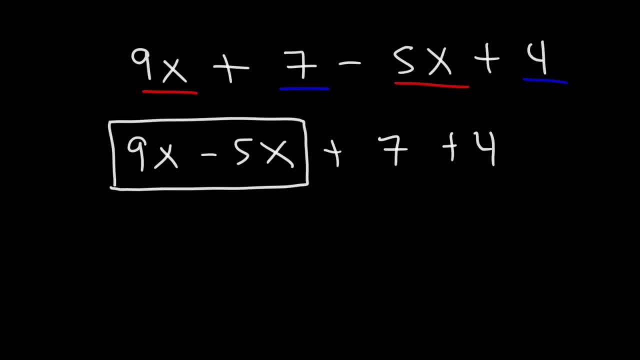 What is 9 minus 5?? 9 minus 5 is 4.. So, 9x minus 5x, It's going to be 4x. Now, combining these two, 7 plus 4, that's going to be 11.. 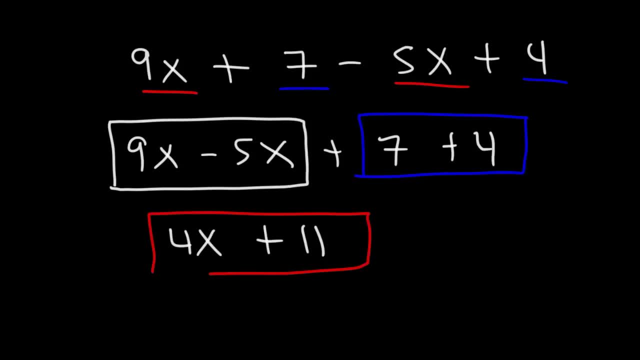 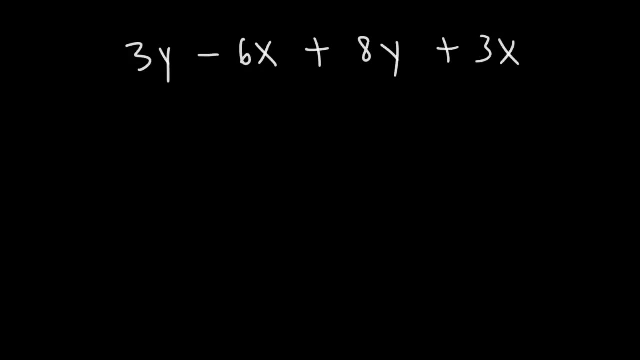 So the final answer for this problem is 4x plus 11.. Now let's work on another example. Let's say we have 3y minus 6x plus 8y plus 3x. So go ahead and simplify this algebraic expression. Feel free to pause the video if you want to. 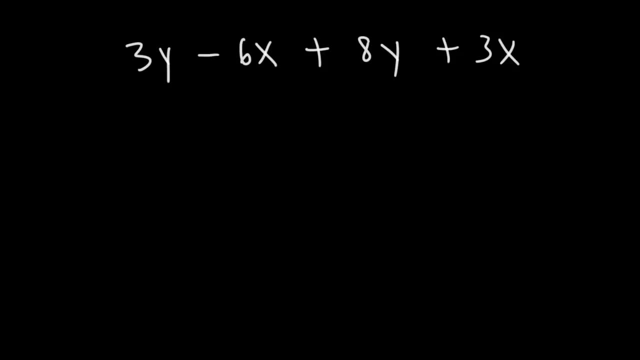 So let's begin by identifying which terms are like terms. So these two are like terms because they contain the y variable. Negative 6x and 3x are like terms. Now you don't have to rearrange the expression. if you don't want to, At this point you can simply combine the like terms. 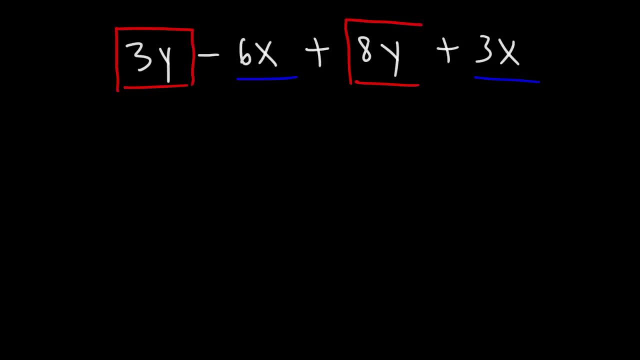 So let's combine 3y and 8y. 3y plus 8y is 11y. Now let's combine the other two, So we have negative 6x plus 3x. So what is negative 6 plus 3? Negative. 6 plus 3 is negative 3.. So negative 6x plus 3x is negative 3x. 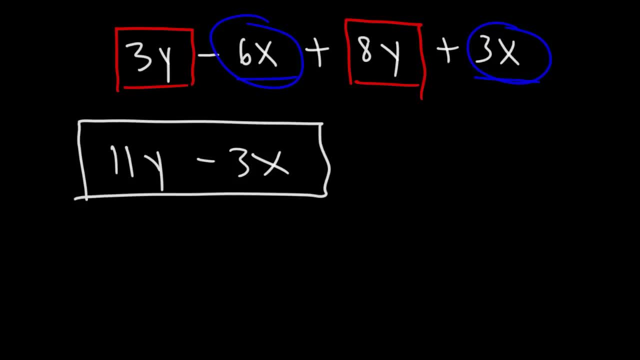 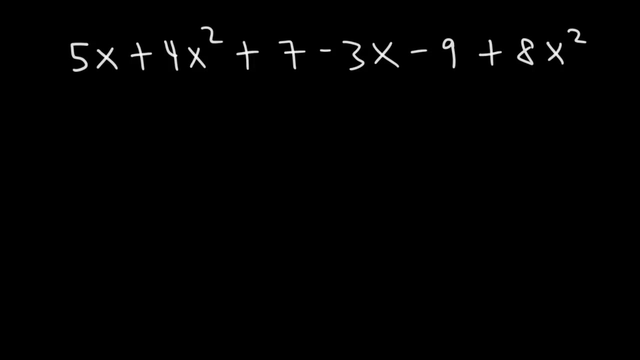 So the answer is 11y minus 3x. Now let's try an example that contains more terms. So we have 5x plus 4x squared, plus 7 minus 3x, minus 9 plus 8x squared. Feel free to pause the. 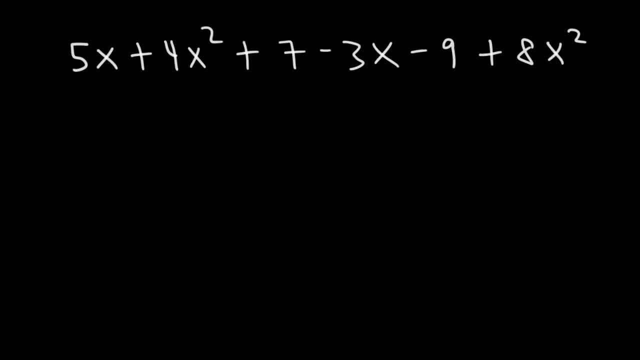 video and work on that example problem. So identify the like terms: 4x squared and 8x squared are like terms. 4x squared plus 8x squared, that's going to be 12x squared. Next we have 5x and negative 3x. They're like terms as well. So 5 minus 3. 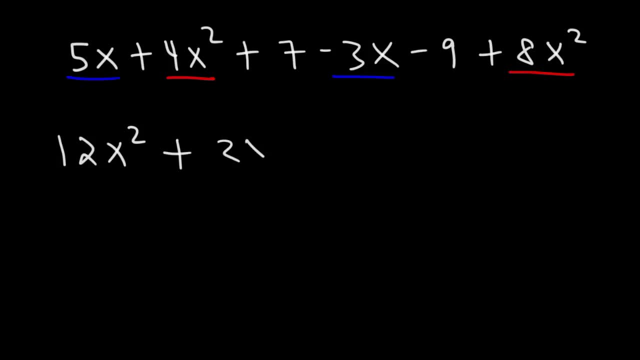 is 2.. So that's 5x minus 3x is going to be 2x. Next we have 7 and negative 9.. Those are the constant terms: 7 plus negative, 9 or 7 minus 9. that's negative. 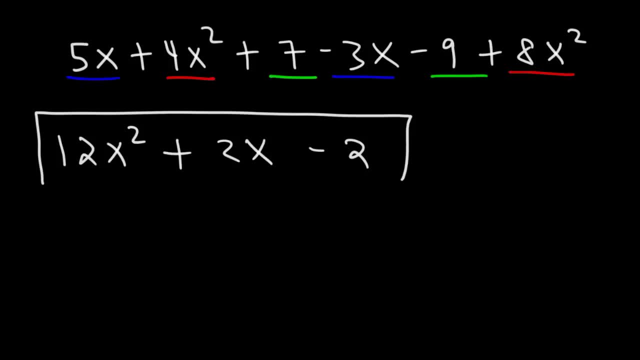 2. And so this is the final answer in its simplified form. So as you get, you can see, combining like terms is not very difficult. But sometimes, instead of having just one variable, like x you may contain, you may have a problem with multiple variables, One containing x and y, like this one. So let's say we have 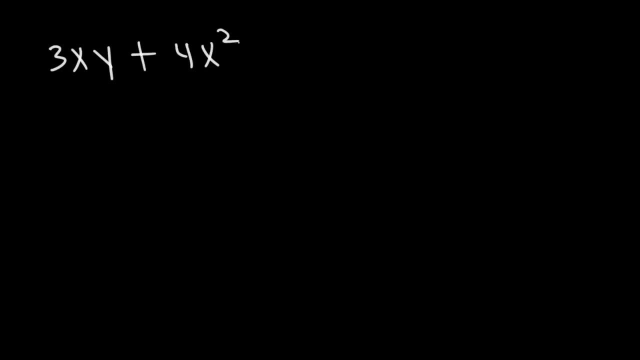 3xy plus 4x, squared y plus 5xy minus 6x, squared y plus 9x. Now this problem may be a little confusing, but don't let that get to you. Focus on which terms are similar. Notice that these two are like terms because they contain the same. 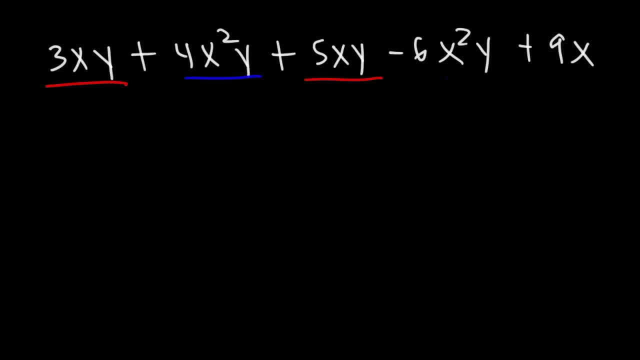 variables x and y. Now, even though these two contain the same variables, they contain the same number of those variables, That is, they both contain an x squared and a y, So they're similar to each other, but different from x- y. Now the 9x is by itself. So let's say, we have x squared and y squared. Now let's 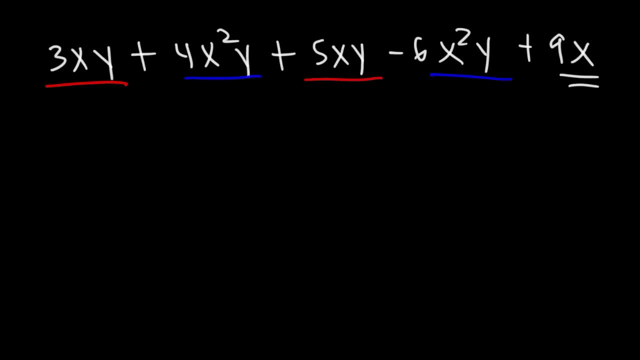 focus on these two. 3xy plus 5xy, 3 plus 5 is 8.. So this is going to give us 8xy. Next we have 4x squared y minus 6x squared y. 4 minus 6 is negative 2.. So this is: 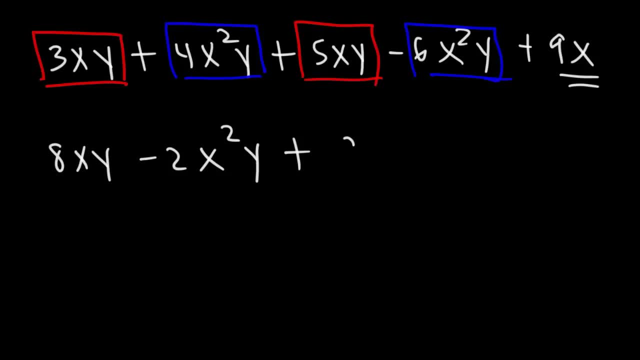 going to be negative, 2x squared y, And then we could just rewrite the last one, since there's nothing we can do with that. So this, right here is the answer: 8xy minus 2x squared y plus 9x. Now what? 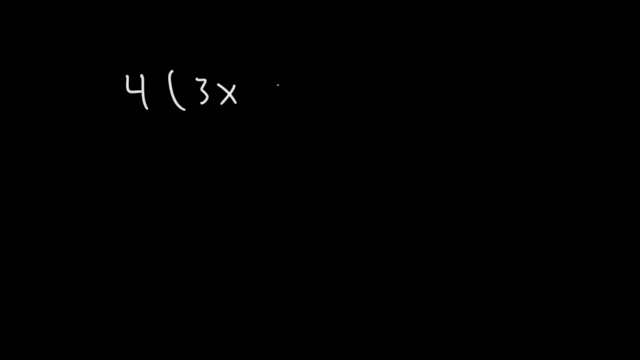 would you do if you saw a problem like this? Let's say we have 4 times 3x plus 5 minus 7x. Go ahead and try that Now. if you have parentheses, you need to use something called the distributive property. We need to distribute the 4 to. 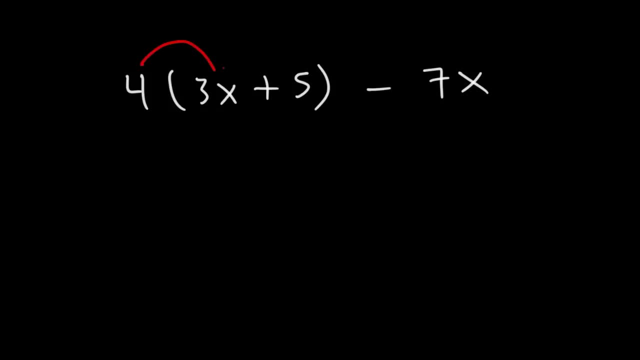 3x and 5. Use multiplication. So 4 times 3x, 4 times 3 is 12, thus 4 times 3x is going to be 12x. Next we have 4 times 5,. 4 times 5 is 20.. 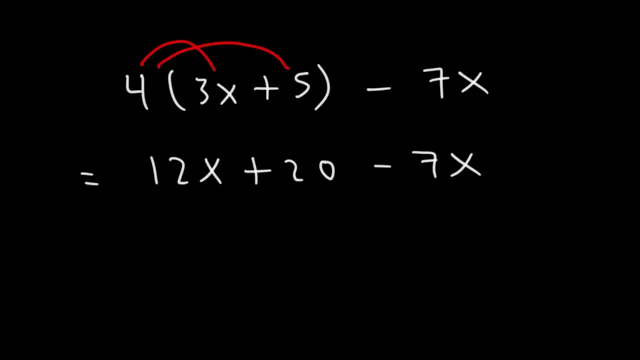 And then we can rewrite this expression on the right. Now, at this point we can combine like terms. So the only like terms that we can combine in this example are 12x and negative 7x. 12 minus 7 is 5, so this is going to be 5x. 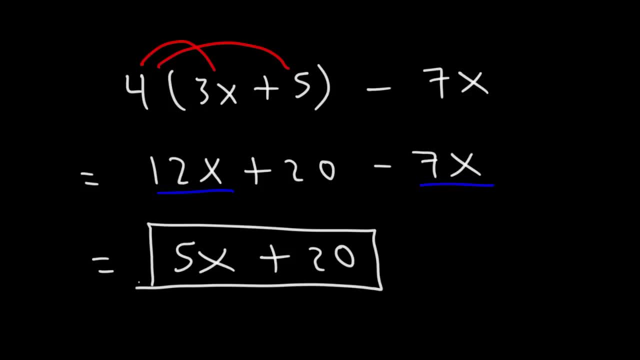 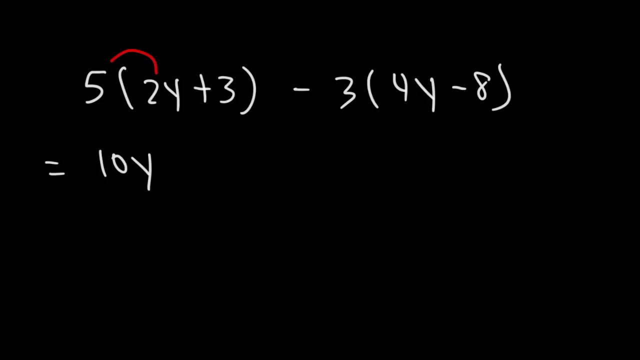 Thus the final answer is 5x plus 20.. Here's another similar example. Here we have 5 times 2y plus 3 minus 3 times 4y minus 8.. So go ahead and try that: one 5 times 2y, that's going to be 10y. 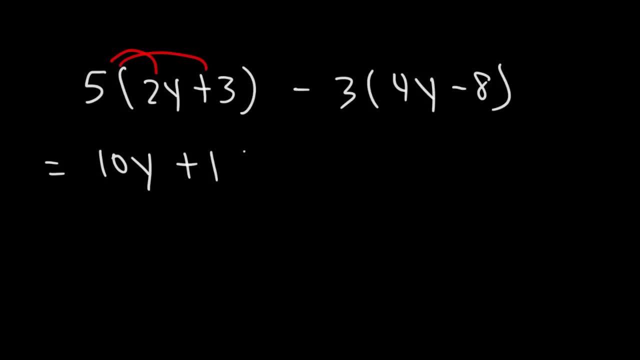 Next we have 5 times 3,, which is 15.. And then negative 3 times 4y, that's negative 12y, And negative 3 times negative 8,, that's going to be positive 24.. Next we need to combine like terms: 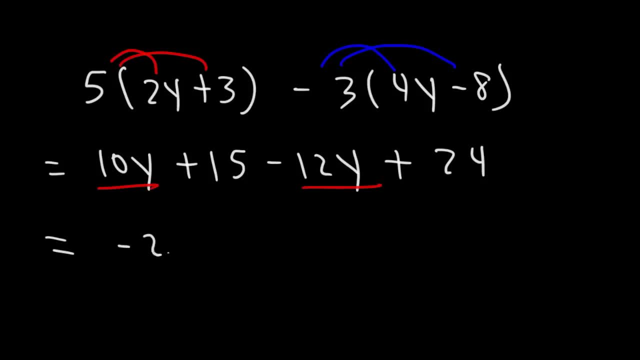 So these two are similar: 10y minus 12y. that's negative 2y, And then 15 plus 24.. That's negative 2y, That's going to be 39, positive 39. So the final answer is negative 2y plus 39.. 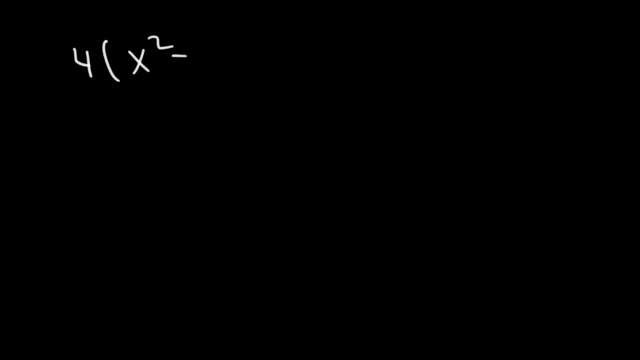 Try this one: 4 times x squared plus 3x minus 5, minus 5 times 2x squared, minus 4x plus 7.. So first we have 4 times x squared, That's going to be 4x squared. 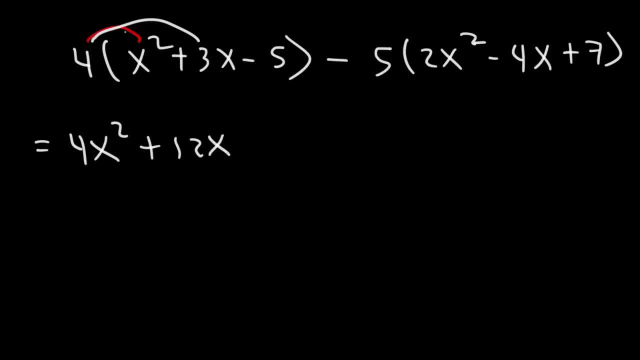 And then 4 times 3x, That's 12x, And then 4 times negative 5,, that's negative 20.. Next we have negative 5 times 2x squared, That's negative 10x squared. And then negative 5 times negative 4x. 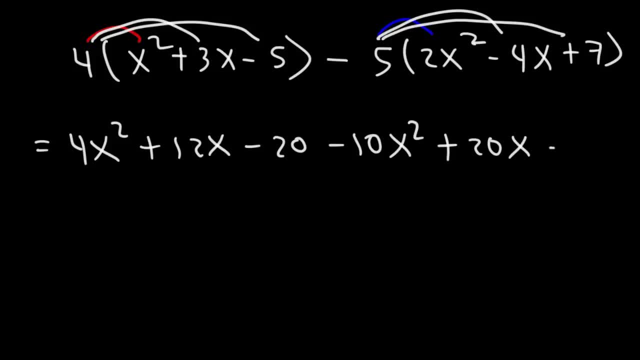 That's positive 20x, And then negative 5 times 7,, which is negative 35.. By the way, if you feel that I'm going too fast, you can always pause the video and try this yourself. All right, So the next step is to combine like terms. 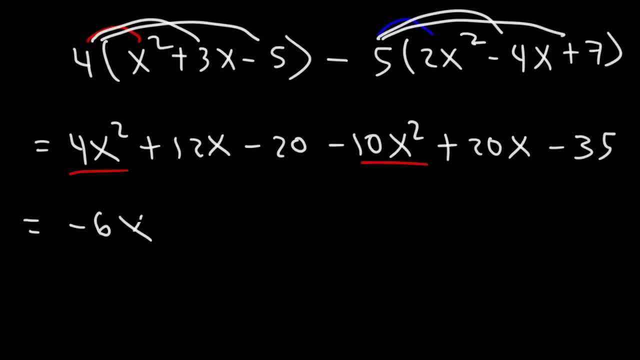 So these two are similar. 4 minus 10 is negative 6.. And then just write the x squared on top of that or to the right of it. Next we have 12x plus 20x. That's going to be 32x. 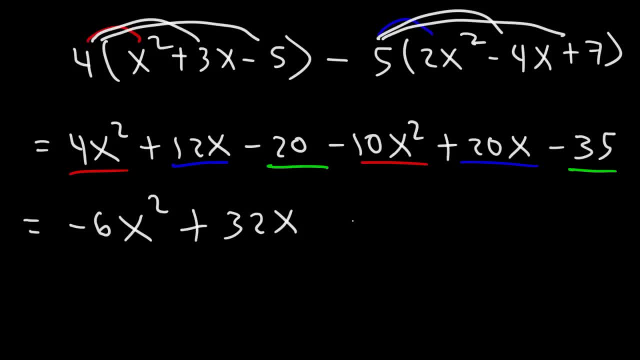 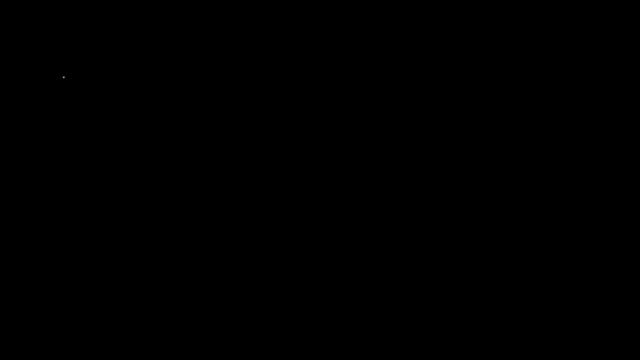 And finally, we have negative 20 minus 35,, which is negative 55. And so that's it for this example. That's the answer. Let's work on one more example. So we have 3 times x cubed plus 5x minus 8..